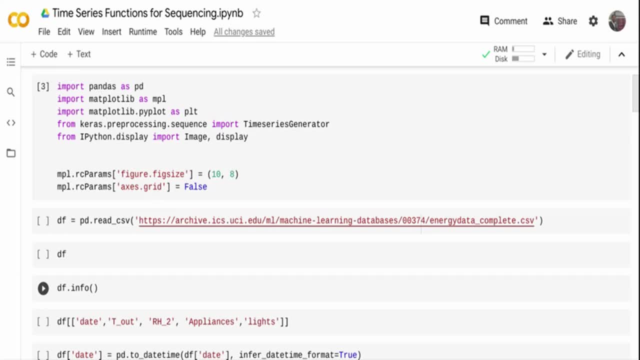 Hi, in this video I'm going to focus on data, preparation of time series, data for sequence models- sequence models like LSTM or RNN, or even other neural network models like ANN or auto encoders. So this is a very important step when we start using deep learning models. Basically, in deep learning models, you need to pass data in a certain format, And what we are going to learn here- how we can prepare the data so that it can be easily fed into neural network models. 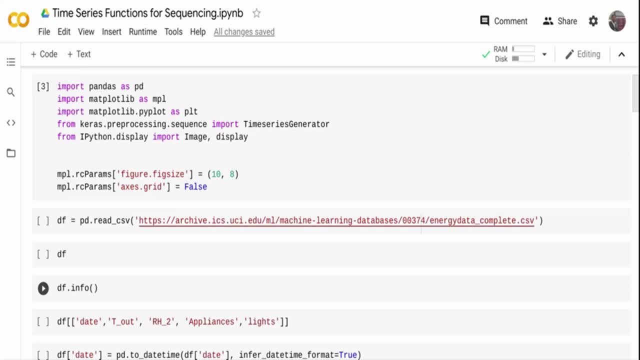 And I'm going to cover the modeling part in the next video, but this is purely focused on data preparation. We will also see different time series, concepts like sliding window and hopping window, which are also based. So let's get started. So what I'm doing is I'm importing Pandas library matplotlib for visualization and I'm using a package called Keras preprocessing sequence from Keras preprocessing sequence. 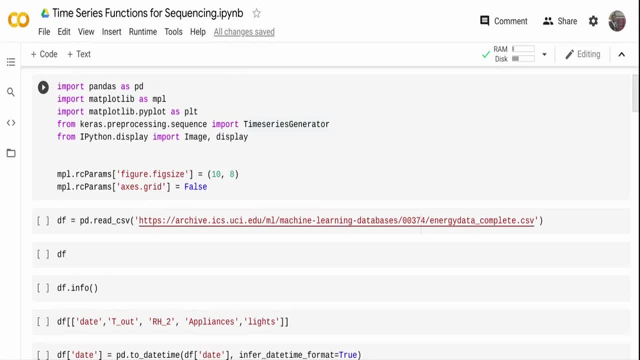 I'm using time series generator. While you can use your own functions to prepare your data, there's a very handy function which simplifies the way you can prepare the data for neural network models. I'm using time series generator and I'm just using iPod. 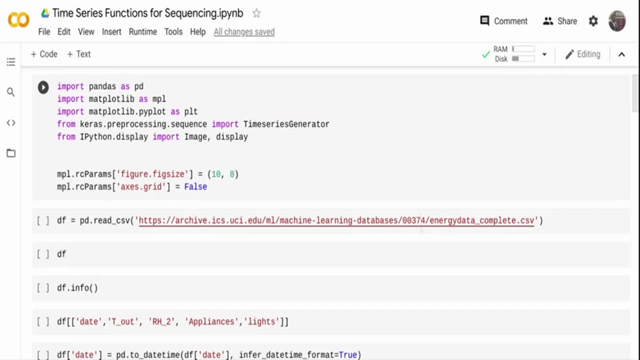 And I'm going to show you some examples of how the data is prepared. So let me run this one, and then I am importing a data file from UCI repository. So basically, this is an energy consumption data. It has data of energy consumed by various appliances. 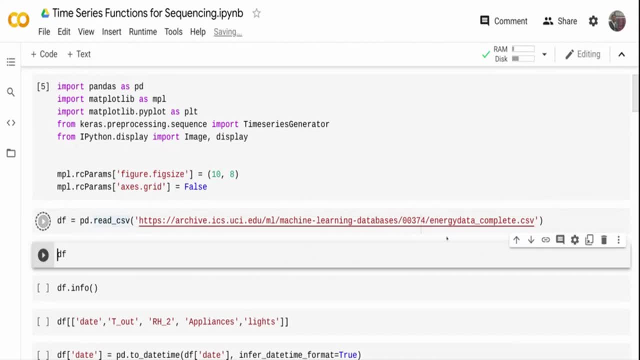 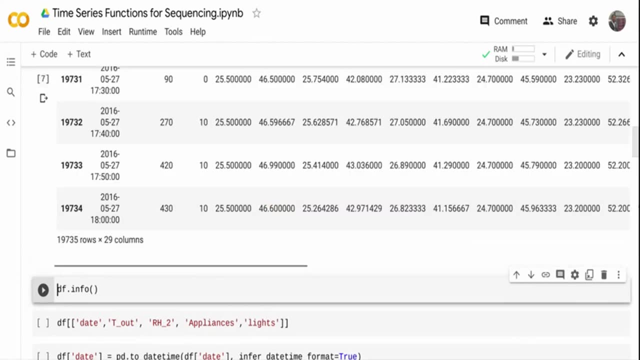 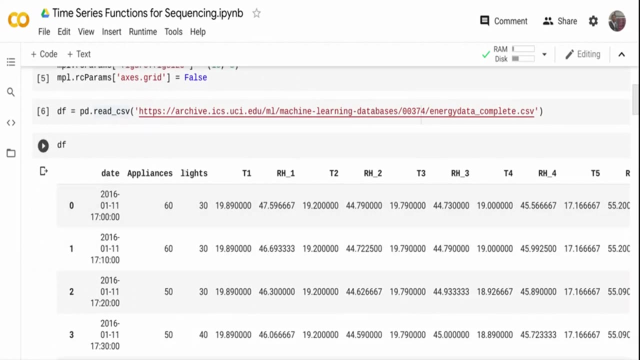 So I'm going to read this particular file. You can get the file from UCI machine learning repository. If you see that this data, There are a lot of features in this data over here. So basically you can see, the first column is the energy used by appliance, the energy used by light on a particular day. 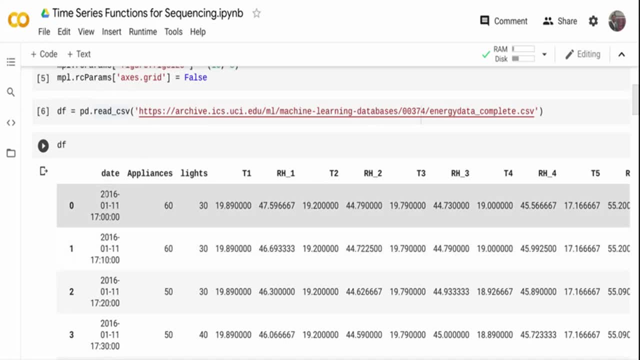 And this data is set at 10 minutes interval. So you can see data at 5 o'clock, 510,, 520, 530.. So every 10 minutes we have data over here And there are a lot of features over here. 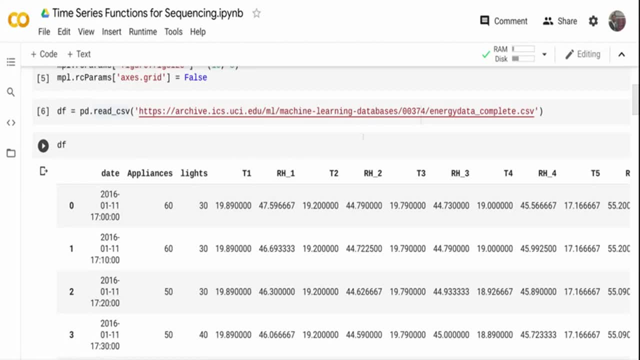 You have temperature in the living room, humidity in the living room, temperature in the kitchen, humidity in the kitchen, And for this purpose I'm going to show you how to prepare multivariate data for your sequence models, But I'm not going to use all the features. 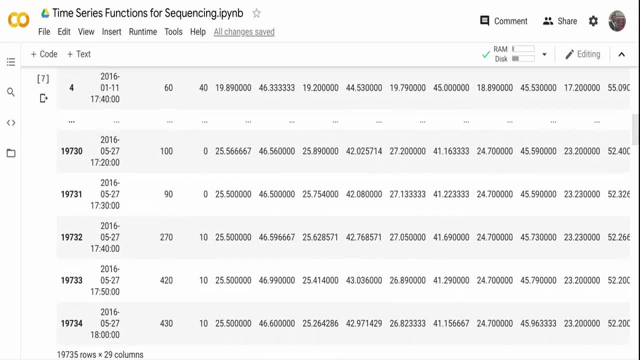 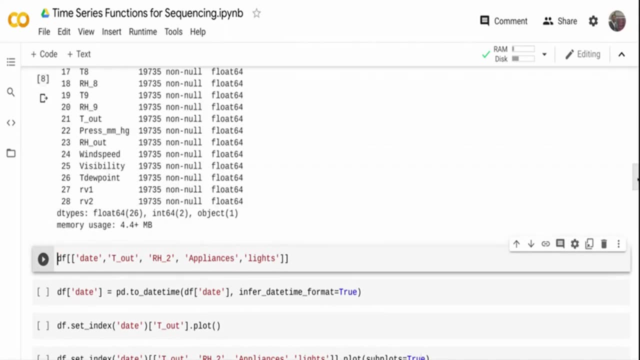 I'm going to use some three or four features on it. I'll focus on that for now. So let me quickly get the info of this particular data frame And you can see like there are a lot of columns. There are 28 columns. 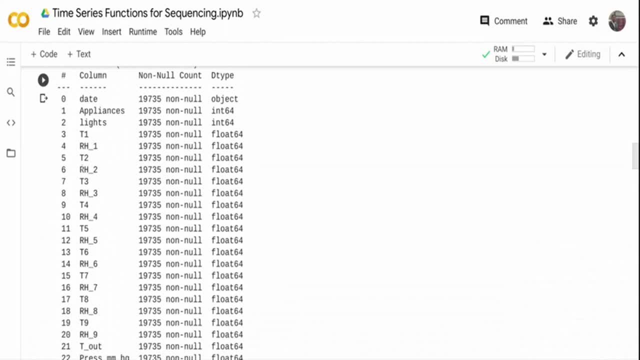 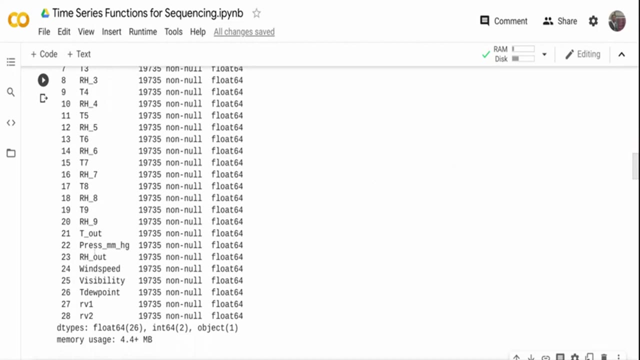 You can see, like temperature and humidity, the temperature and humidity for each and every room in that particular particular house where this particular appliance usage is captured. You then also have the outside temperature, which I'm going to use. You have outside pressure, humidity, outside wind speed, visibility. 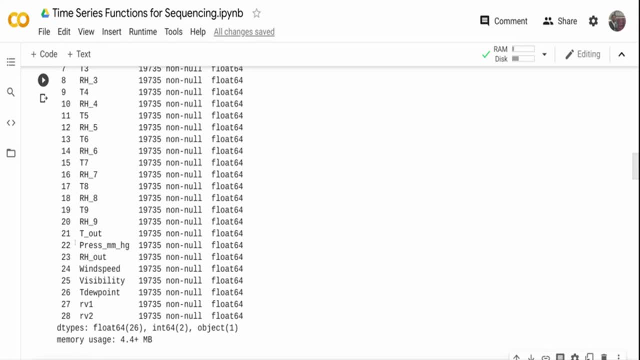 So what we are going to do is we are going to prepare data in such a way like: maybe based on the outside temperature, pressure, humidity, Can we predict the appliance energy usage? That's what we are going to do. We are going to prepare the data for that. 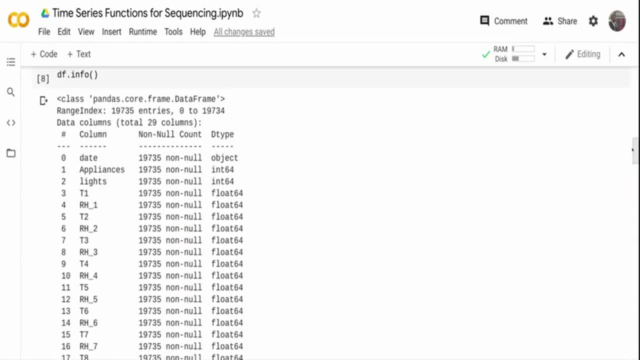 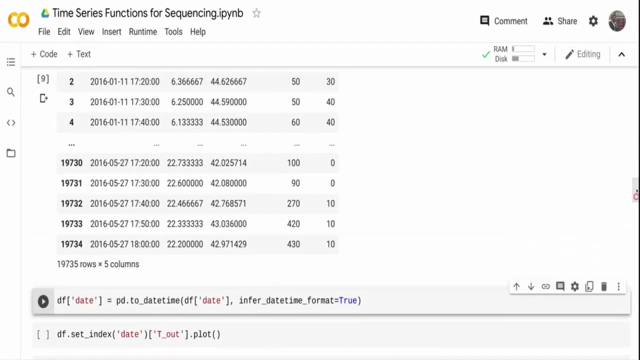 So what I'm going to do is Let there is also a date column which, you see, the date is object and for the analysis for some of the time series and as we need to convert this date into timestamp format, So what, what I'm going to do is I'm going to use these columns for this particular video. 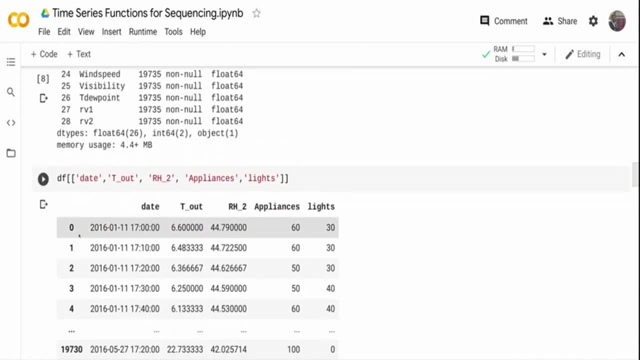 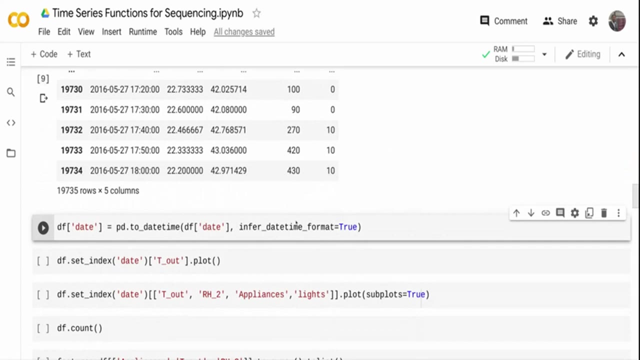 The columns are basically the date, the date when the particular reading was captured, the outside temperature, the outside humidity, appliance energy usage and lights energy usage. I'm going to more focus on Appliance energy usage, Right? So first thing I need to do is I need to convert the date column into a timestamp format. 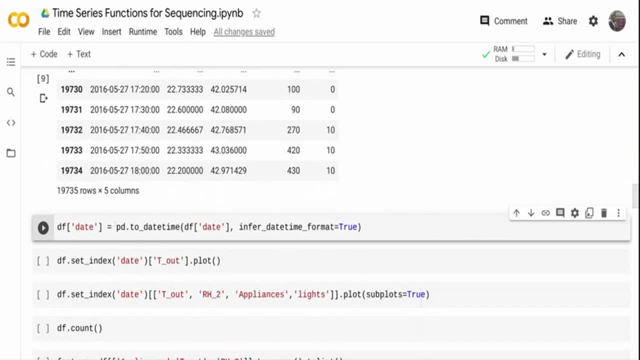 So what I'm doing for that is, I am taking the date column, I am converting, using Pandas, to date and function, passing the data and telling him for the date format. So once I have this date format, I can quickly plot the plot, the output. 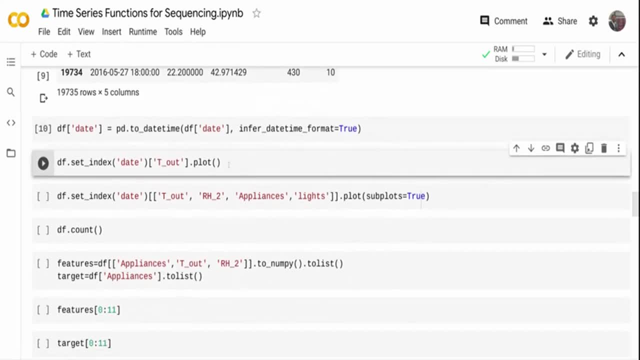 Right. So for plotting the temperature output for column, what I am doing is I'm telling like the data frame, I'm telling the time series as index. So if you have data index, you can use a lot of time series plots that are available by default in the Pandas function. 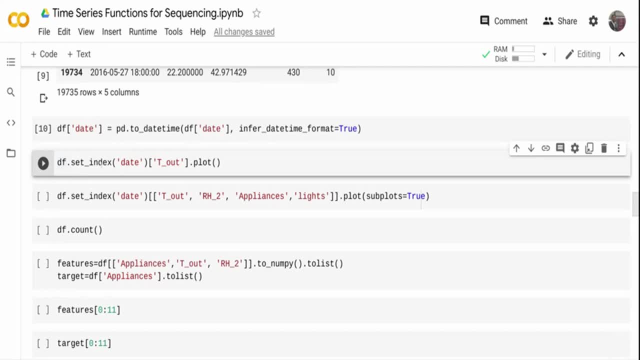 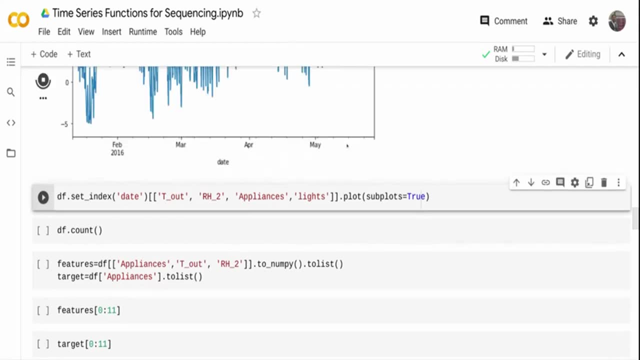 Right. So basically it will always be your exacts if you set it as index. So I'm setting the index as data, I'm taking the temperature out column and I'm just doing a plot. So if you see what it's going to show, the plot of temperature. 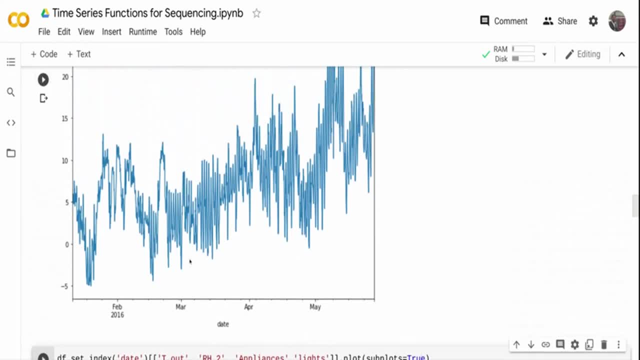 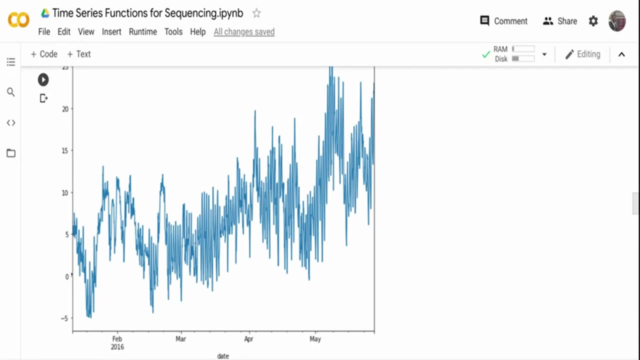 So we have data for February 2016 to May 2016.. You can see, this is how the energy usage is and the energy usage is constantly increasing Over time And basically, maybe, if you take a rough assumption right during the February month and March month, the temperature are typically not that hot and it's either like just out of winter or spring, and you can basically see that the appliance usage is lower. 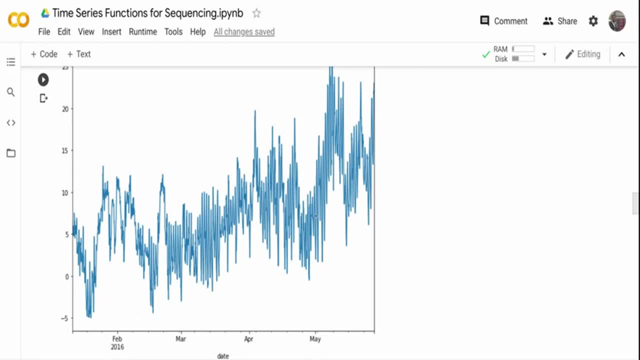 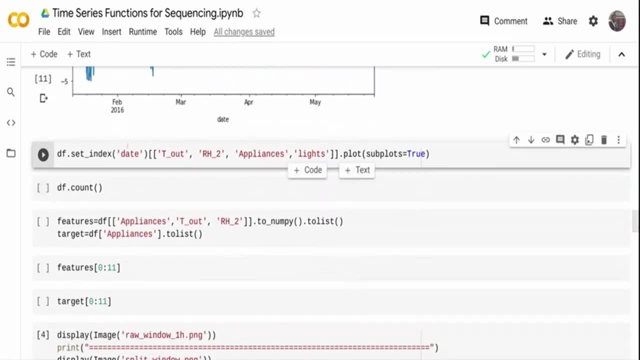 The temperature is lower, but the temperature steadily increases during the month of April and May. So that's what we are seeing now. We can also plot all the metrics together to see How they are correlated. So in this case, I am setting the index as date. 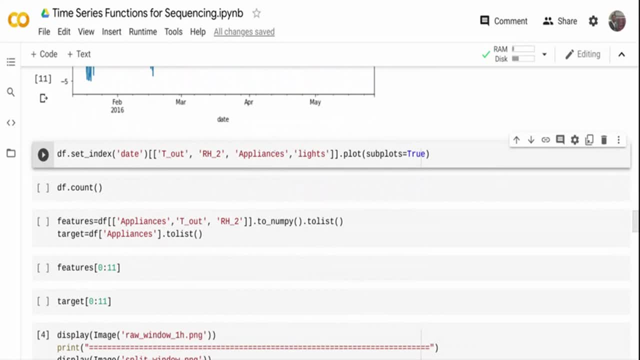 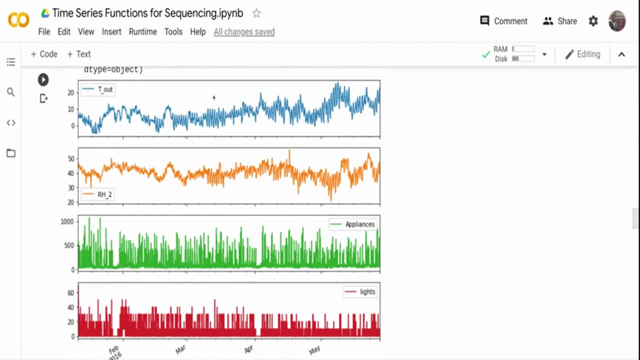 I am using temperature output, humidity appliance and lights and I am creating a subplot for each. So if you, if you see over here in this plot right, we saw already the temperature. the temperature is basically, uh, during the February month the temperature is low. 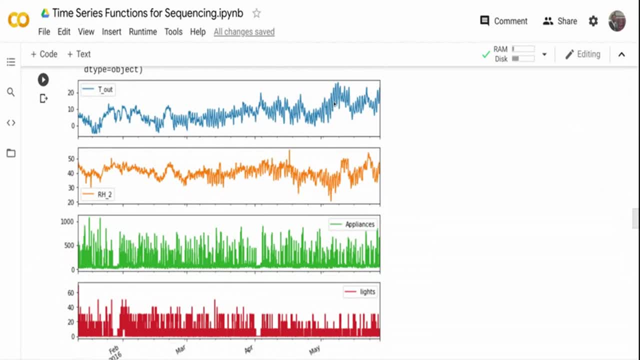 It's typically winter and then it starts increasing during the summer and the humidity also like kind of follows the temperature pattern to some extent. But if you see the appliance usage, the appliance, This uh usage is kind of higher uh during the winter month, uh during the earlier February month. 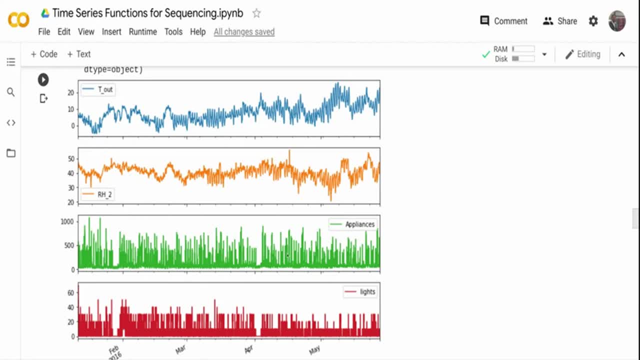 And then after that it's, it's, it's kind of like uh uh, not as high as the winter month, but it's still like there are some peaks you can see in the appliances and even the lights you can see is higher during the winter month. 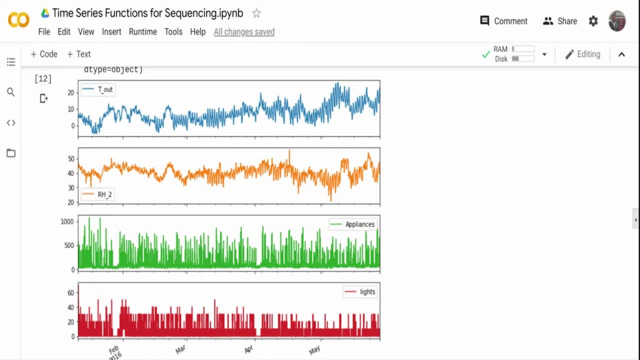 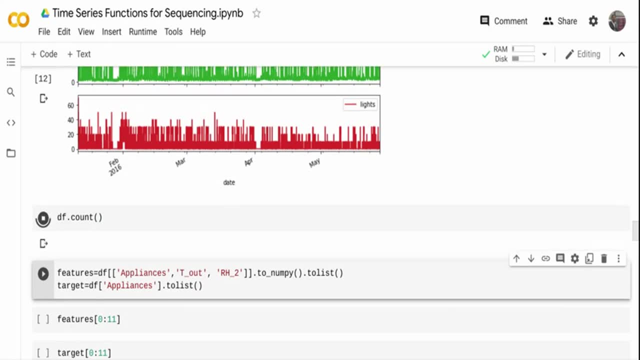 And during the summer it's lesser, because the nature lighting outside during the summer is pretty good, right? So this is the plot right now. Let's quickly do a count of it And you can see there are on 19,735 rows uh in, uh in this particular data set. 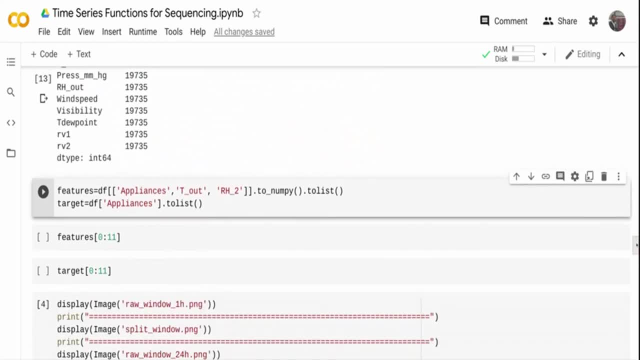 Now what I'm going to do is I'm going to create two uh data frame: the feature data frame and also the target data. I mean the feature data frame. I am using appliances to output temperature and humidity as the feature and in target, I am just using appliances. 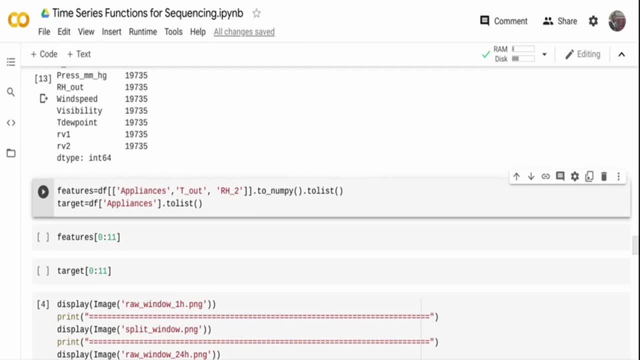 So the idea is: given the current uh appliance usage count for today, the outside temperature and the humidity, Can I predict how much is the appliance usage tomorrow? That's the problem we are going to kind of solve. So just to uh, just for it to use in the time series generator. what I'm doing, I'm converting both into a list. object: 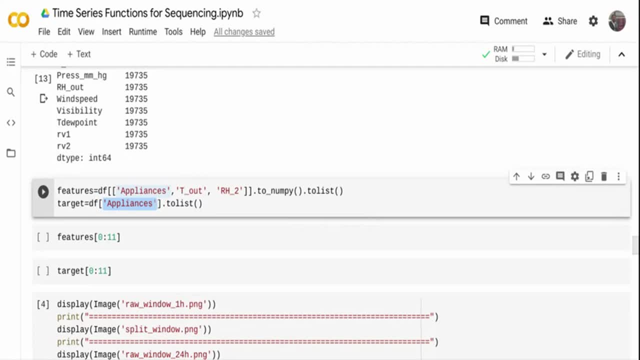 So since in this has only like one data frame column, I can directly call to list. but here I have three columns I cannot directly convert to list. I have to first convert it to a numpy array and then to a list. So now I have the features column and I have the target column. 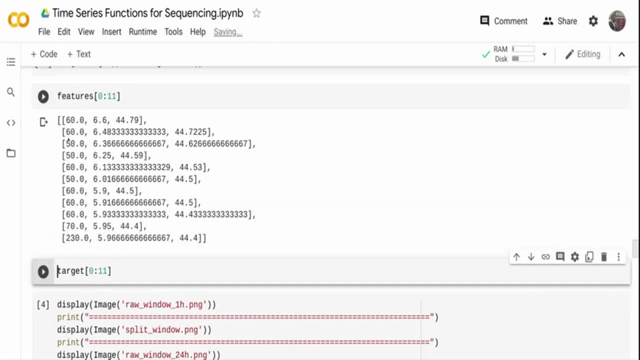 I let me run the first 11.. Uh, rows of the features column. You can see there's a list object. Uh, basically, this was the appliance count, This was the temperature output, This was a humidity. It is basically a list. 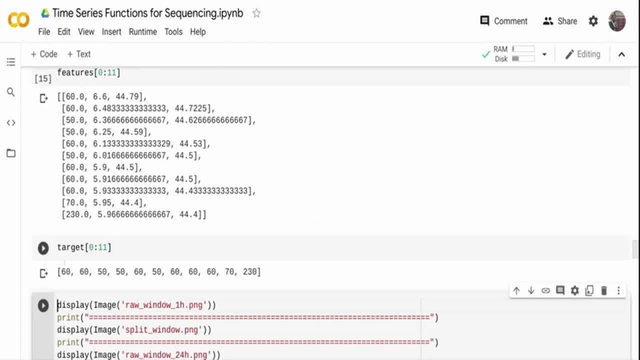 And then the target column output will have uh the, uh the appliance, uh usage, energy usage. So it is 60 Watts, 60 Watts, 50,, 50,, 50, like that. right, You have that. 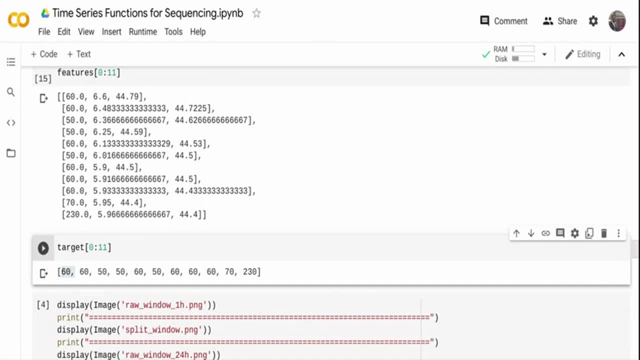 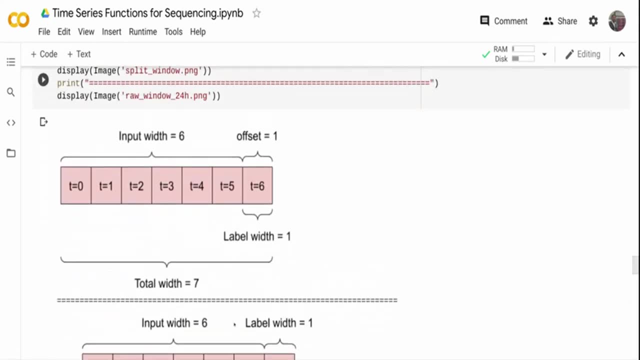 Now what I'm going to do is I'm going to prepare this data so that we can feed it into the sequence model. before that, Let's understand some uh time series concept. So these are images that I've taken from uh, the TensorFlow website. 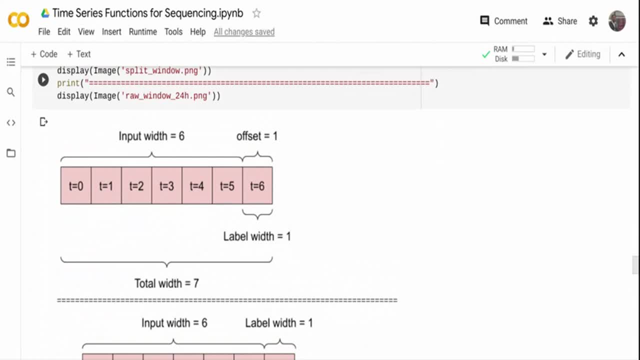 Uh, so, uh, when the you can go and find about these images over there. So the very first thing, what I'm going to do is I'm going to uh take the previous six observation. in our case, the observations are 10 minutes. 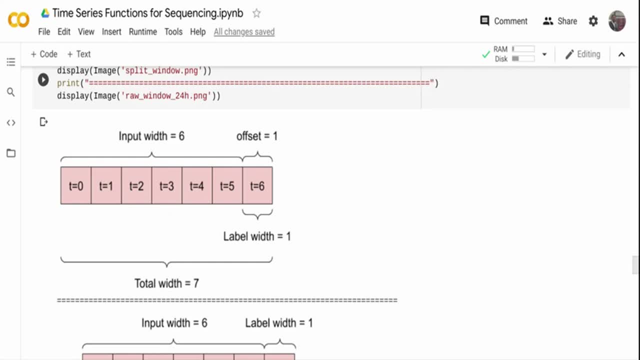 So when I say six observation- in this case that is 10 into six is 60 minutes, That is one hour. So I'm going to take the one hour observation and, uh, predict the next value. So that's what you can see here. 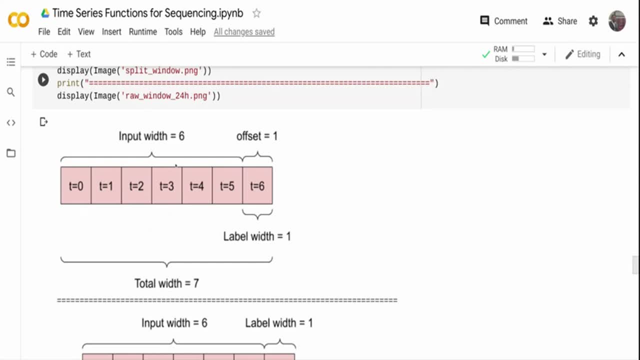 So Okay, So I'm taking time zero to time six value, the input with over here is six, and then I am predicting this next value, That is, the sixth value or the seventh value, because it starts from zero index. So basically that's what I'm doing here. 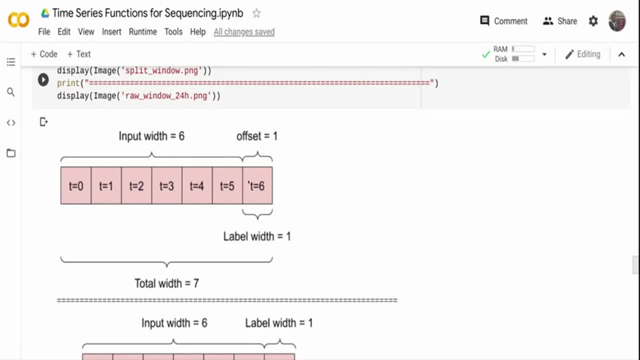 The offset is also one, because we are immediately predicting the next value that we are going to get. So when you talk about time series, like if you are feeding into LSTM model, you need to. you need to basically combine the T zero to T five as an uh. 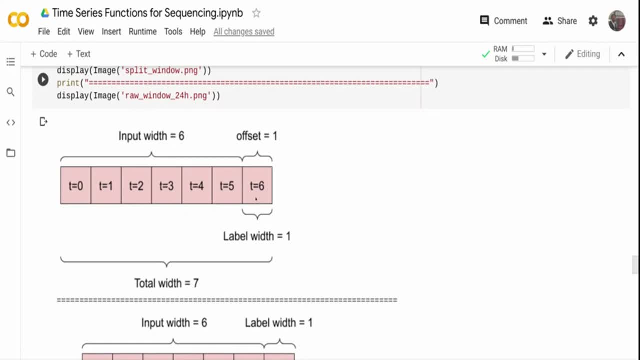 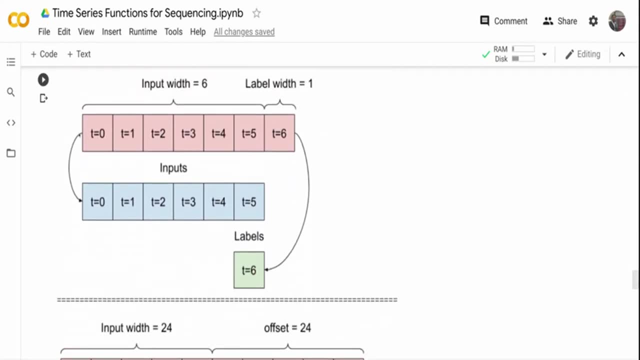 as a sequence to predict the T six which is going to be our label. This is one option, right, The same thing. it's shown here Also. basically, I have time series: T zero to two six, T zero to T five are my inputs and T six is the label. 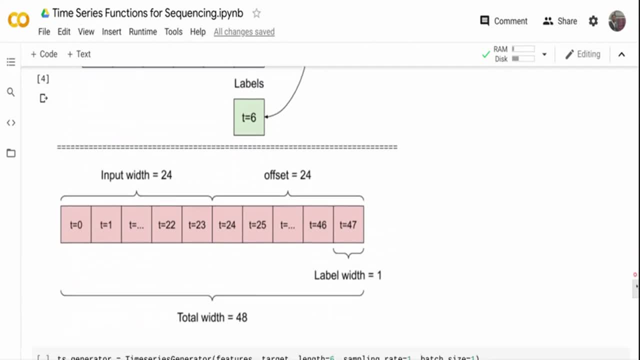 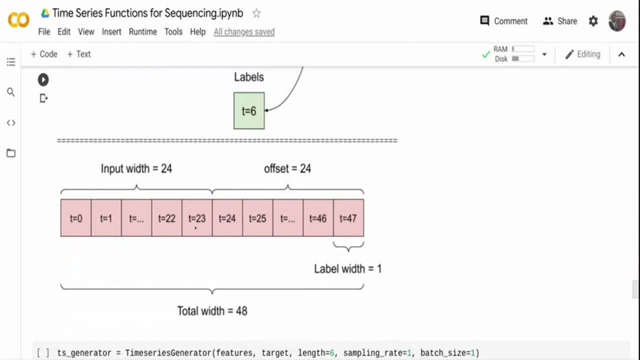 This is how typically you prepare for LSTM. That can also be a possibility where you take the data T zero to T 20, 23, that is a one day data T zero to T 23.. And then I am predicting next day at T 20.. 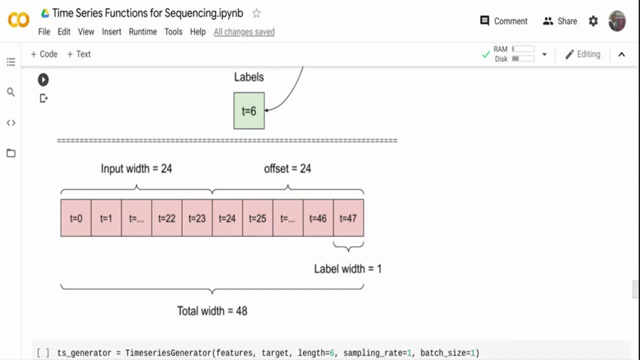 23,. what will be the temperature or what will be the appliance usage? So in that case, if you see the input with this going to be 24,, because I have from zero to 23 observation, that is a day worth of data maybe- or in this case, I have 24, 10 minutes data, as you would send a hourly data rate. 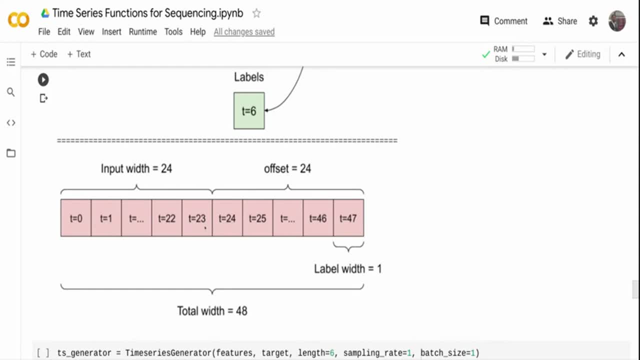 So I have, uh, I have like input with 24, and then what I? what is going to happen? because I'm going to predict only the 47th value right The next day at now. now suppose, uh, now it's. 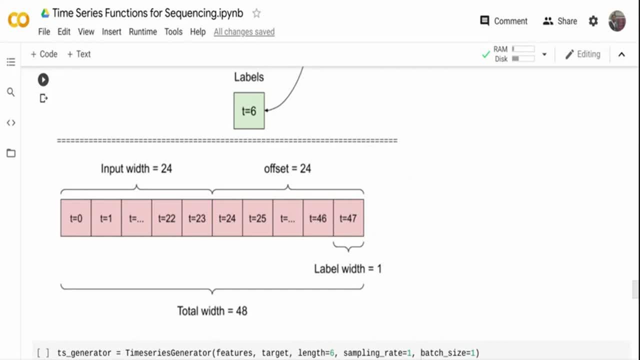 Four o'clock. right, I take the data from yesterday four o'clock to now four o'clock, That is, I have 24 hourly observation. I'm going to predict the value tomorrow at four o'clock, So in this case the offset is going to be 24.. 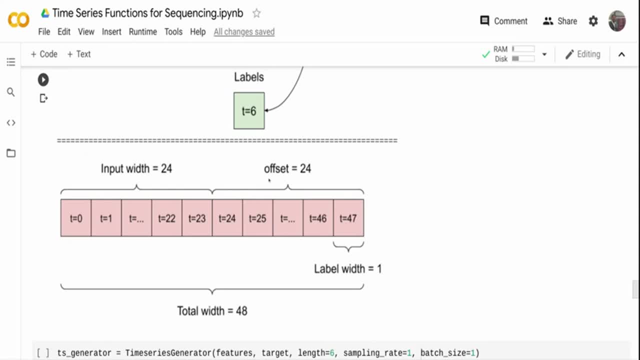 The input width that we are going to pass to the model is 24.. The offset is 24.. The label is at the 47th interval and that is the second format that we have that we can prepare the data for LSA. 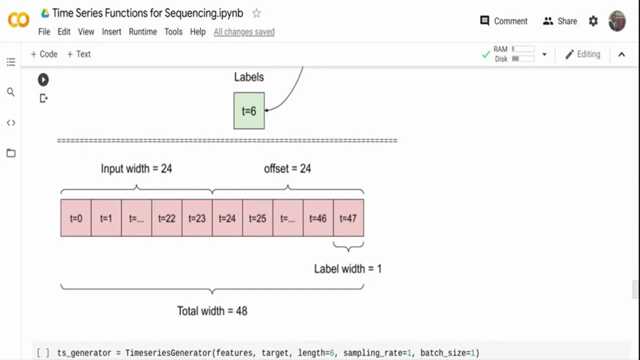 It depends on what is our use case right, Whether we are going to solve Uh, predict the next particular observation, or we want to predict a value somewhere in the future. there can be other way also, where you can have multiple outputs. 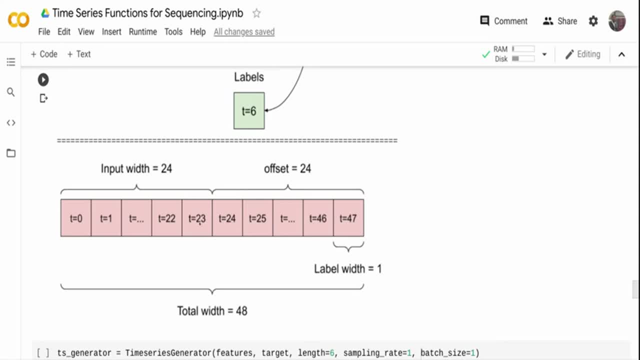 So basically you have, in this case you may have zero to 23, and I want to predict what will be: 24,, 25,, 26,, 27.. So you have multi output in this case, and that is one other option as well. 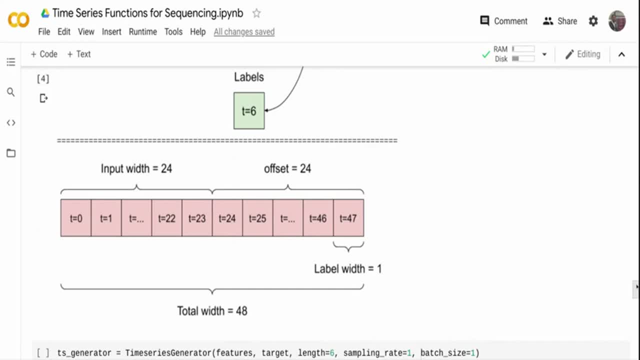 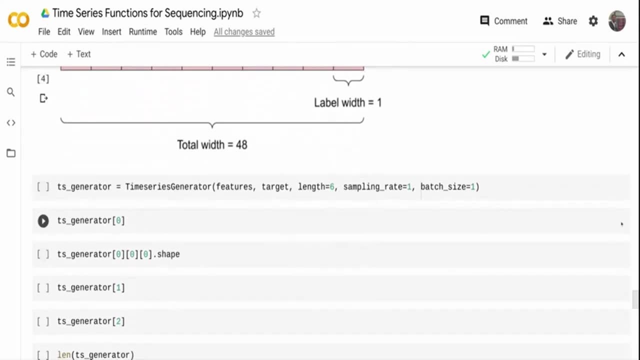 And I will show how to prepare multi output data as well: uh, both multi input and multi output. So now, uh, now what I'm doing? This: I'm using the time series generator to prepare, uh, the, maybe the first format, right? 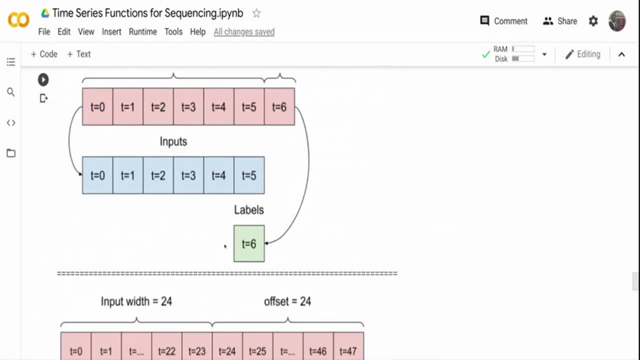 That we saw you'll take the six time series, So seven. seventh will be our label, since it starts with zero. I'm just, uh, skipping the zero. If you take from zero, zero to five will be our observation and six will be our time series. 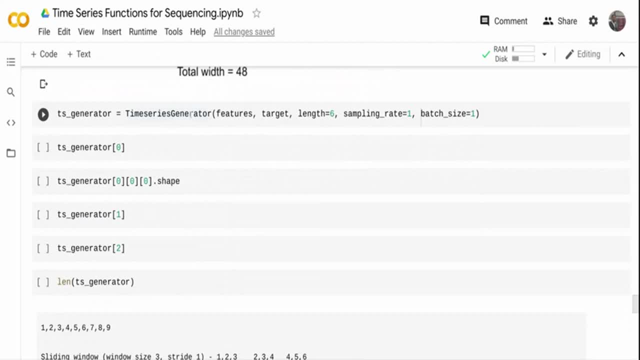 So for that what I can do is I'm using the time series generator. I'm giving my futures input list that I prepared on the top. My future inputs list has three columns. It's a multivariate Uh column that we have. I have a target column, which is again the appliance. I'm telling my length as six. 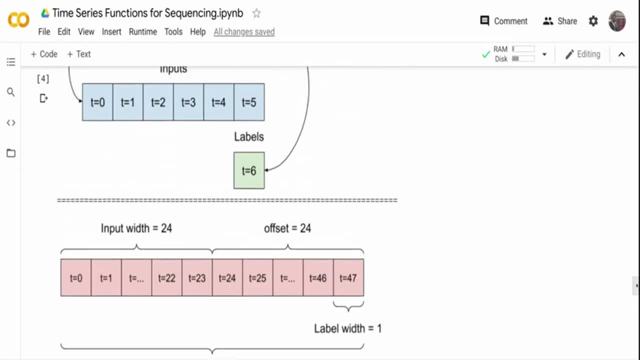 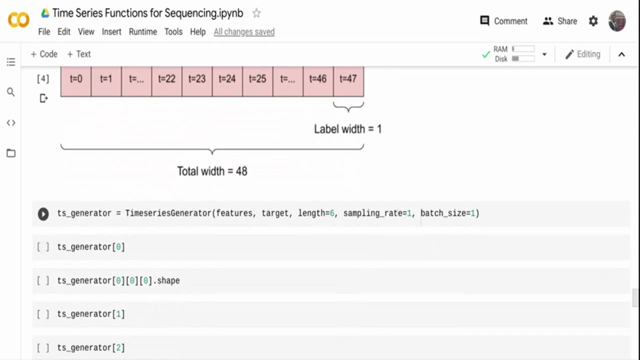 So when I say length as six, that is the input with we are talking about here, the input with over here, the input with this going to be six And then the sampling rate is going to be one. Uh, we are going to just keep the sampling rate over here as one, uh, because we want continuous value. 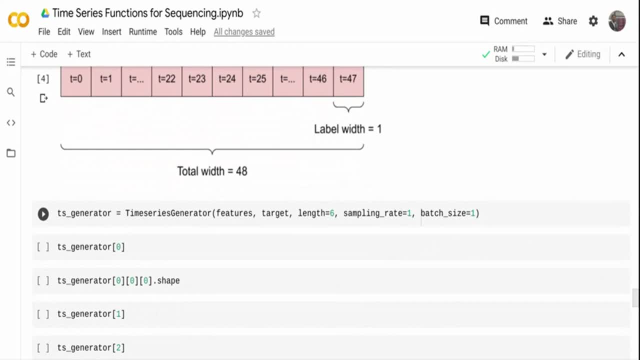 If you don't want continuous value, if you want, like, every third of the time value, then we can use sampling rate three. In this case, we want continuous value And I'm telling batch size equal to one. Now, batch size, you can set it to 64 or 128 when you are training the model. when you are training the model, you don't want to train on lower batch size. 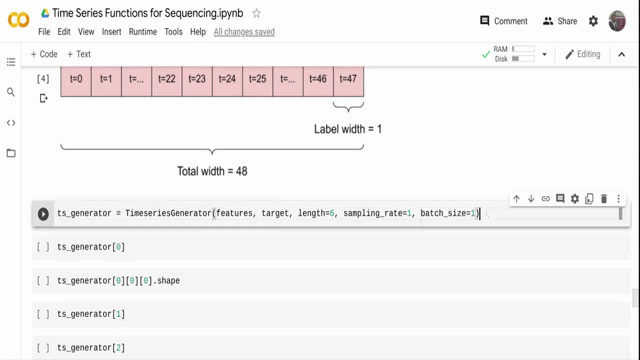 You want to send it in mini batches, right, And that's where you set the batch size. but for- uh, for our purpose, we'll set it as one. So now I have this generator, Let me run the output and see how it looks like, since I have one. 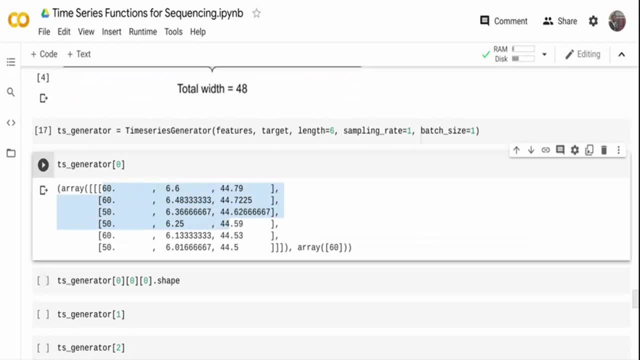 Now, if you see over here, it has taken- this is the input value- It has taken six time steps. I'm giving length. It's equal to six, six right. So basically it's taking like 66.6.. 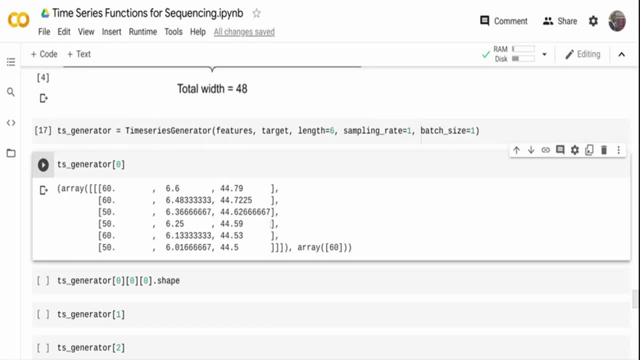 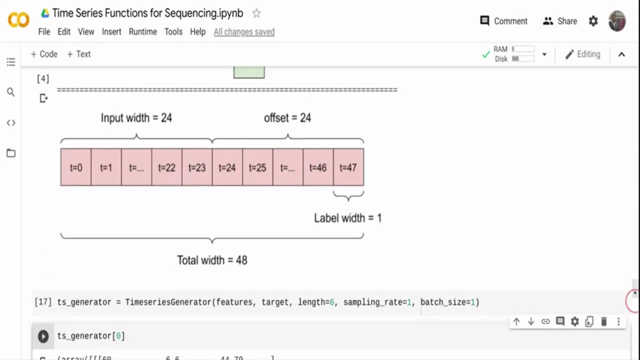 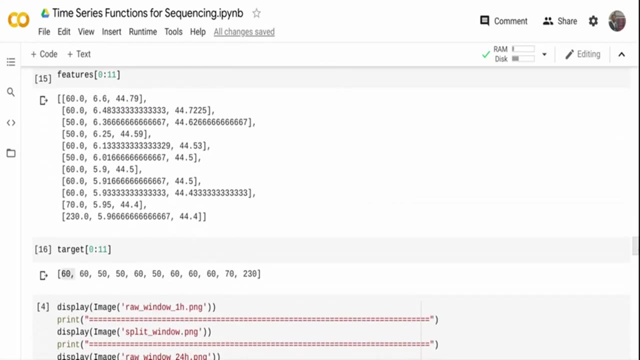 This is the first T0 time step. This is a T1, T2,, T3, T4, T5. And the target is going to be your T6 time step. right, If you go on the top, if you see this particular value that we printed, uh, where we are printing like 11 value C over here. 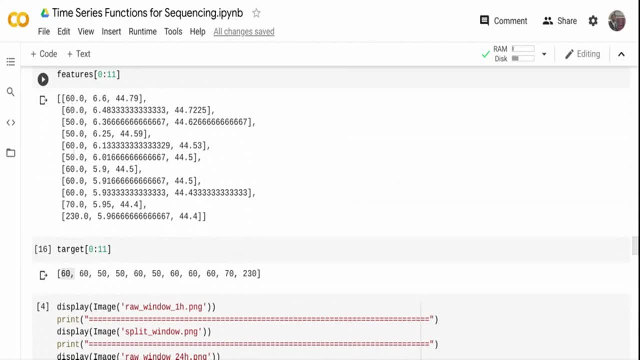 So this is the first time step. second time step: third, fourth, fifth, sixth time step, And this 60 is going to be my target value, The seventh time step. So, given the six value, I'm going to predict with them whether the next value is 60 or not. 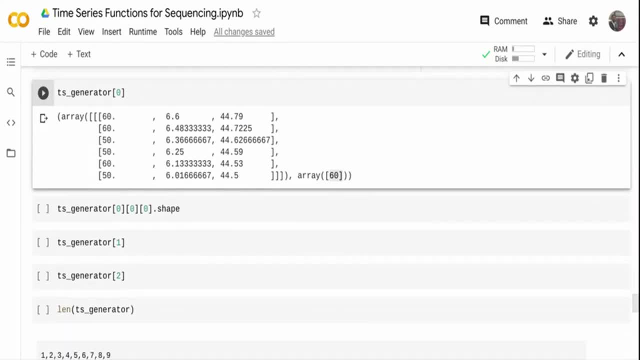 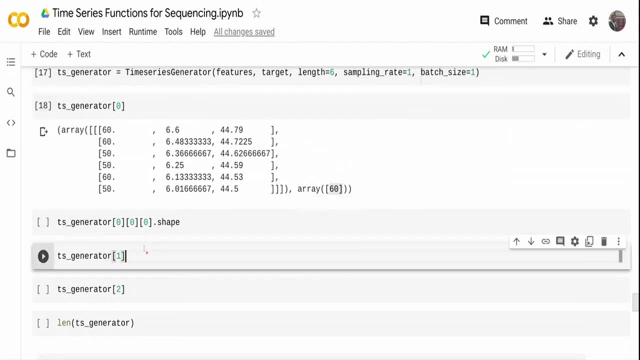 I'm going to train my model such a way, right? So that's what I'm doing over. So this is a one of the option, right? So, since I get the did PS generator of zero, it is giving me the first batch, but if I run one, it's going to give me the second batch, which will be the next 60.. 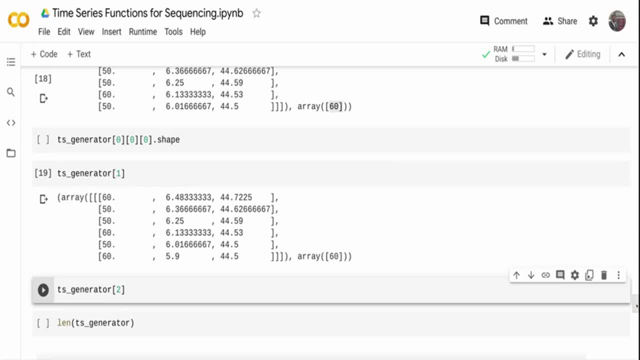 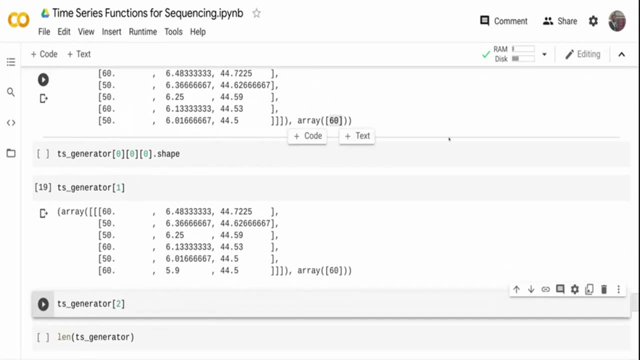 Now this is where another concept comes into play of you want to move the data, whether you want to slide the observation or off the observation. I'll come To that, but what this is going to do is it's going to skip the first row. 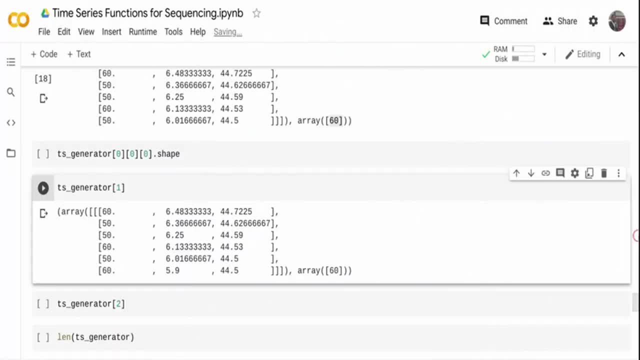 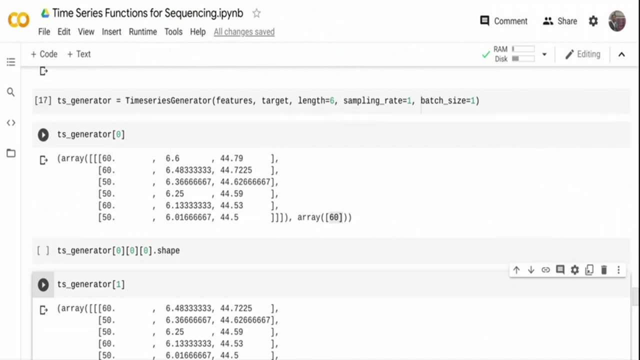 Now, sorry, just a minute. I clicked on this, Yeah. So what it's going to do is it's going to skip the first column. It's going to move the crusher to the second, to a second, to, from that, six columns. 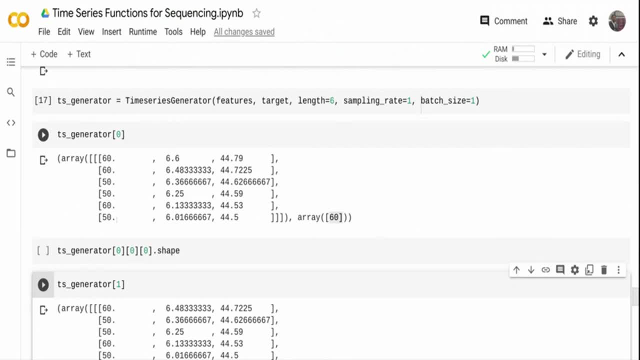 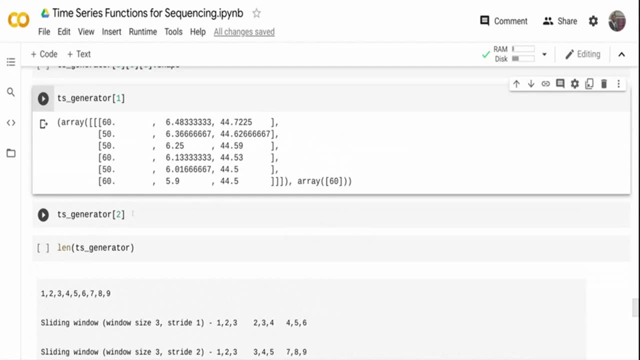 So it's going to be 60,, 50,, 50,, 60,, 650.. And again, the next column was 60. It's going to take that and it's going to run the next value as target. Similarly, when I run, 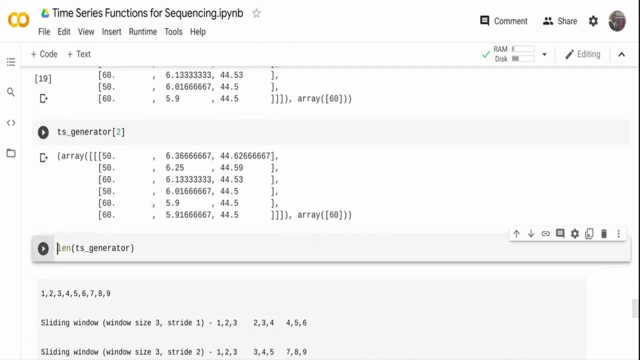 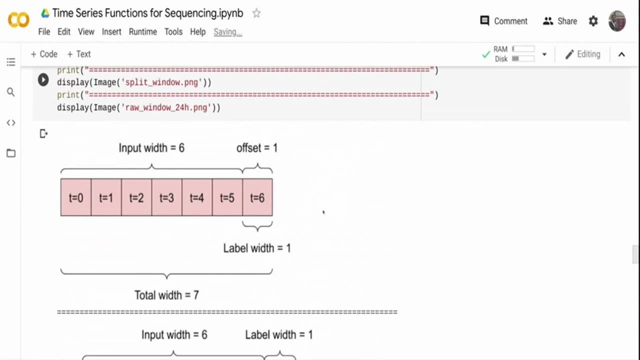 PS generator two. it's going to slide one more window. That's what it's doing over here. So to give the example from the top right, So what it's going to do, if you see, like this was your first batch, the second batch is going to start from T one to T seven and T eight will be your label. 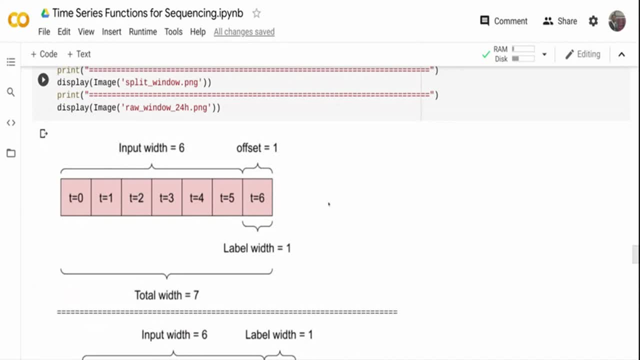 The third batch is going to start from T two to T nine, or whatever T, T two to T seven, and T nine will be your label, or T eight will be your label in that case. So it's going to keep on sliding the window. So that's what is done. 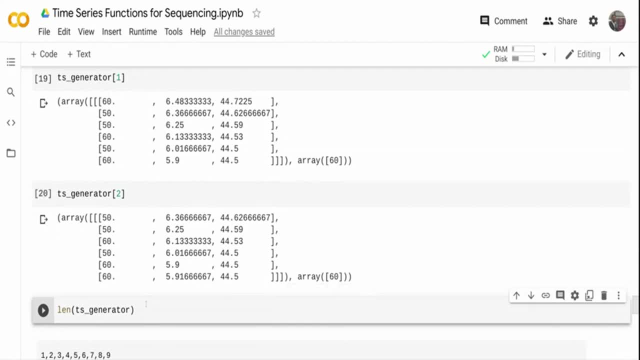 So that's what the batch does. It's going to move based on the batch size. The batch size can be one, in our case, or it can be two, three, four or five, And you can just spin the length of T as generator. 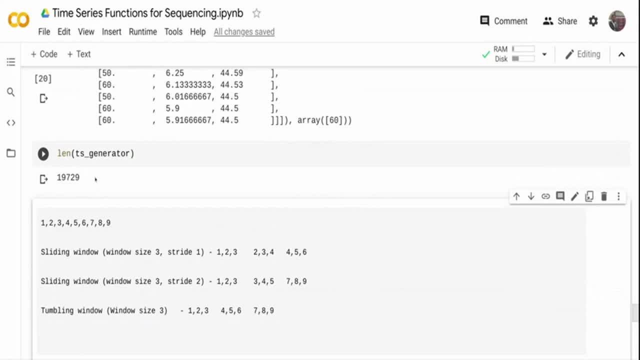 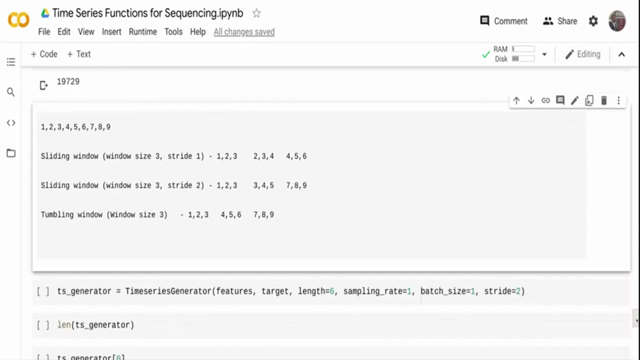 Since I have only batch size one, it's going to be almost similar to the number of column minus six. because the last six value it cannot. it will not have the whole label for that, So it will skip that right. I'll come to that in my next video in detail when I show you, but for now we'll just understand the concept. 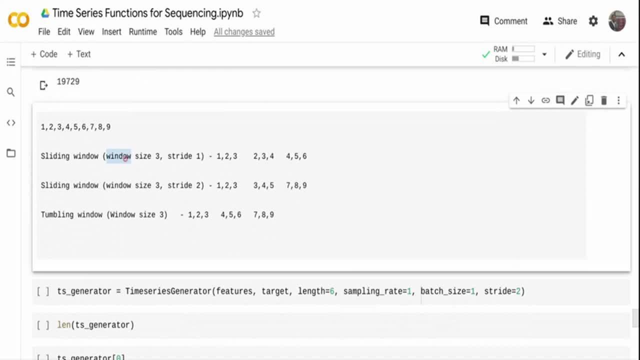 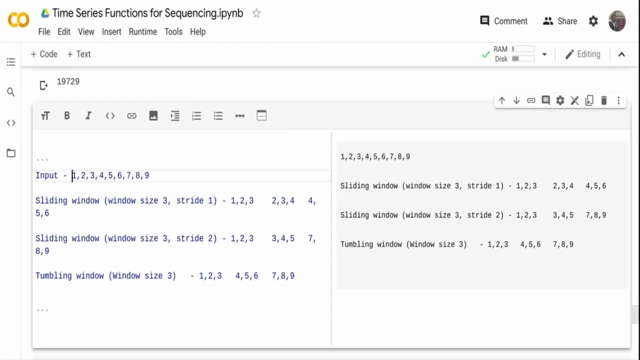 Now let's talk about the sliding window and the tumbling window concept I have been talking about. So, as you, let us assume this is our input. Okay, The input, our input, contains like a one, two, three, four, five, six, seven, eight, nine. 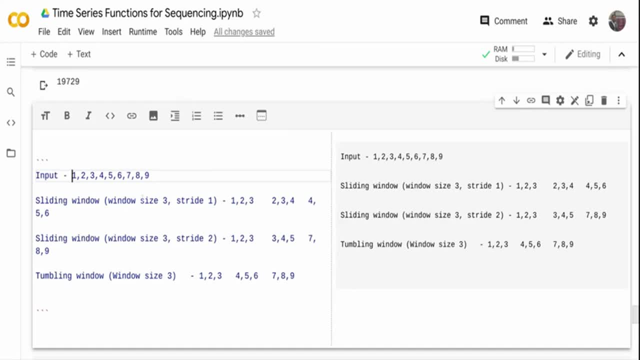 So the sliding window is basically: uh, if you see, I'm giving a window size of three and stride one, right. So the window size three is one, two, three, All right, And then basically I'm telling my stride one. 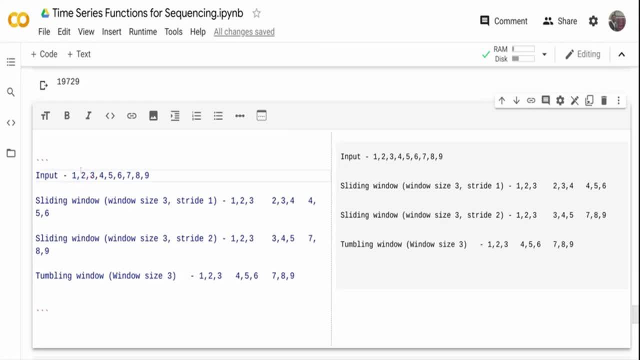 So what is going to happen first is going to take one, two, three. In The second, it's going to take two, three, four. In the third, it's going to take three, four, five. That's what it's going to do. 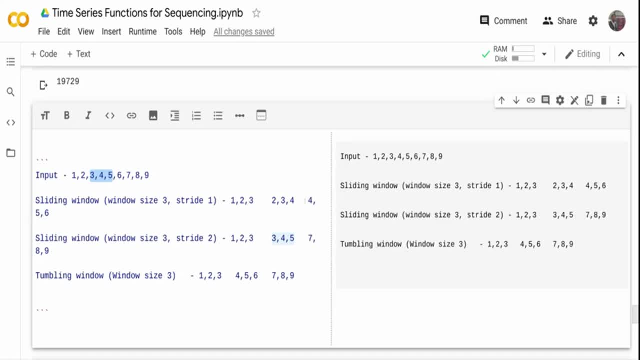 It's going to kind of slide one by one, right, Two, three, four. I I missed three, four, five, but it will be three, four, five and then four, five, six. So on, here it's sliding one time, step by one time step, based on the stride size. 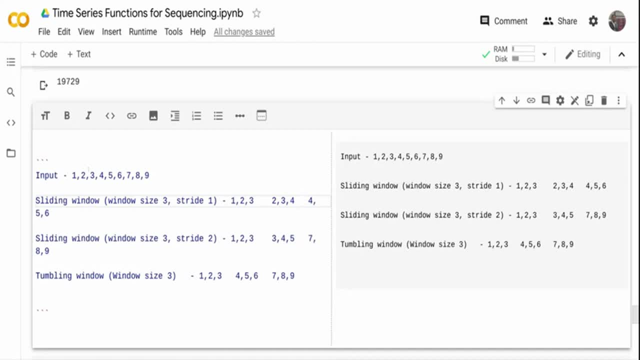 But if I give stride size two, it's going to take one, two, three, and then it's going to skip the two, three, four, because it's going to. I'm telling stride size is two, So first It's. 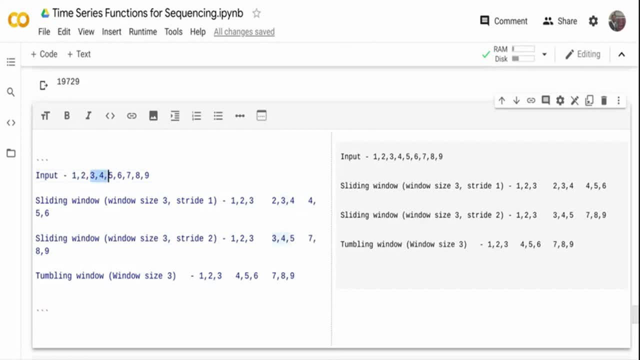 Going to take one, two, three, then it's going to take three, four, five, and then it's going to, uh, take basically five, six, seven, and then it's going to take seven, eight, nine. 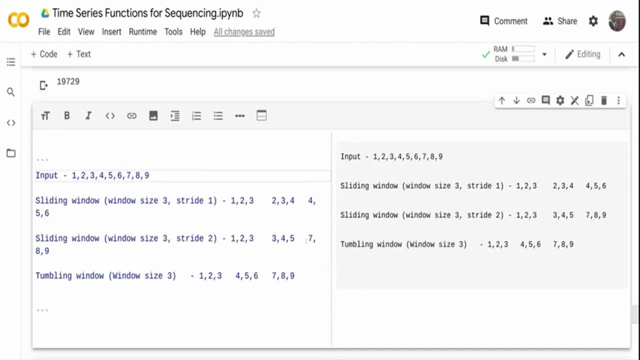 So, uh, I have not put all the observation here, but, uh, that's what it's going to do, right, It's going to stride, It's going to skip one. If you give stride three, it's going to skip two and go to the next. 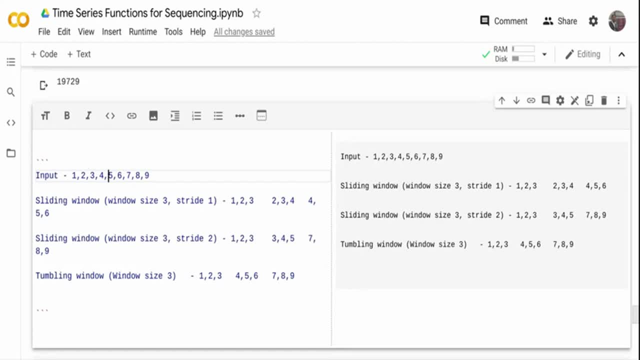 Now this is sliding window right Now. this is very important in your machine learning feature engineering as well. Suppose you are doing some real time analysis on: uh, what Was customer last? uh third last, uh five spends right. 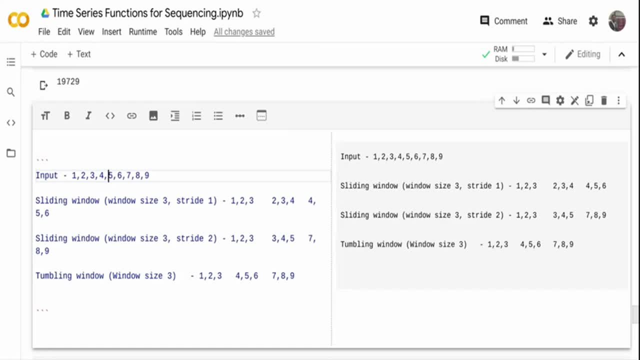 You can, uh, you can either like do a sliding window, like, uh, suppose the customer does a six spend, you will take off the first spend and they'll do do the uh, how much on the next five spend? you keep on like moving. 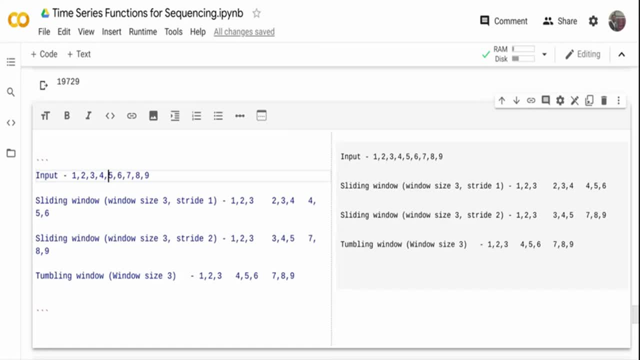 So that the always the window size is fine, right? So that is one option. Hopping is something that you completely skip it. So in this case now it's called hopping window or tumbling window. It can be either way, right. 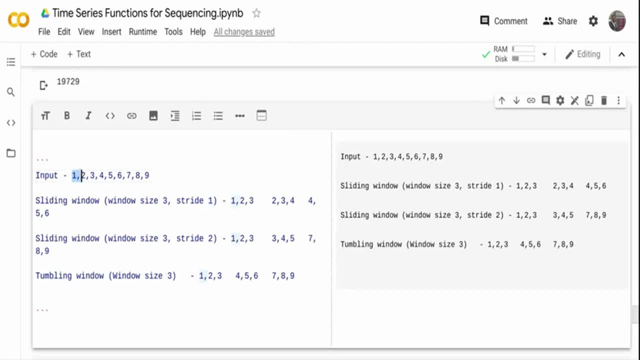 So in this case, Right When I say window size is three, it's going to be one. two, three is going to be the first window, And then four, five, six is going to the second window, Seven, eight, nine is going to be third window. 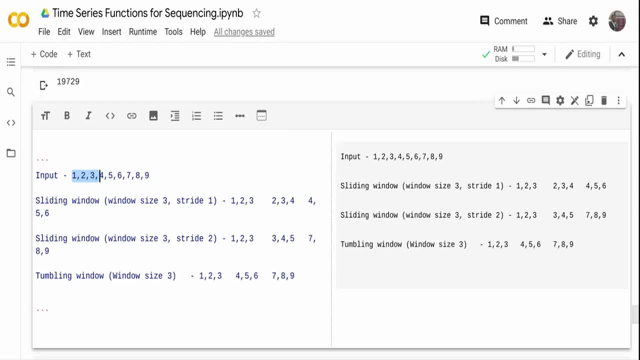 So that is no overlapping here at all. So what it is doing is it is basically hopping, It is skipping the results. So if I always want the latest three count, then uh, I can, I can just use the tumbling window, right? 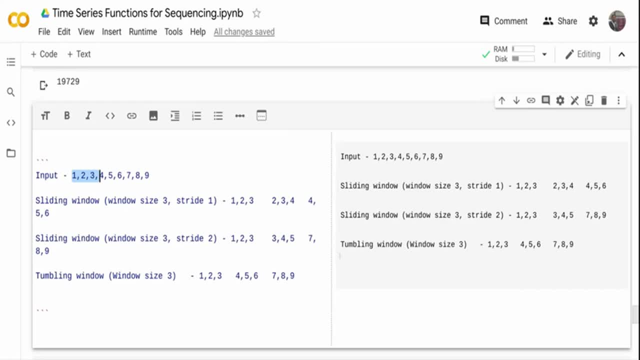 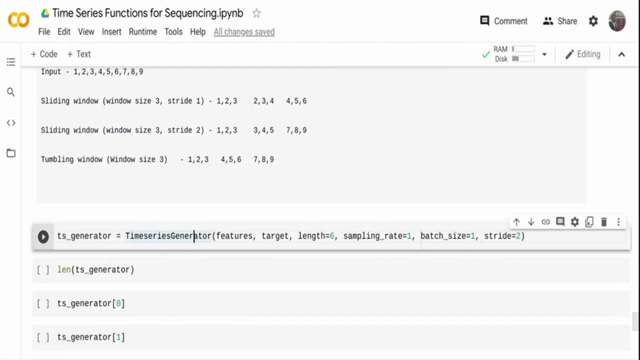 I don't want overlapping windows, Then I can use a tumbling window or hopping window. So this is the other concept. Now let's see how to implement that in a time series generator. It's the same thing which we spoke about, but in this case what I'm doing is I'm adding a new parameter called stride two. 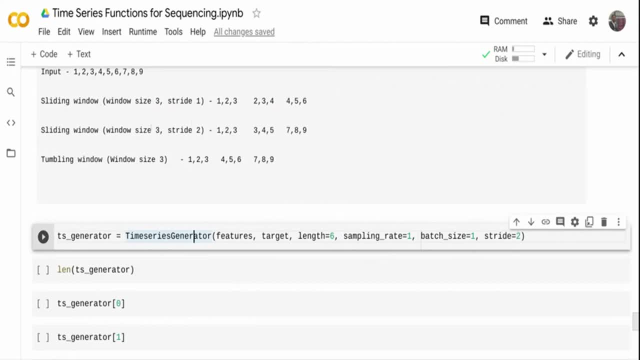 If I want to implement the second one right With the window size of six. So here I'm telling my features: my length is six, The sampling rate is same, batch size is same, but my stride is two. So this will give me a generator over here. 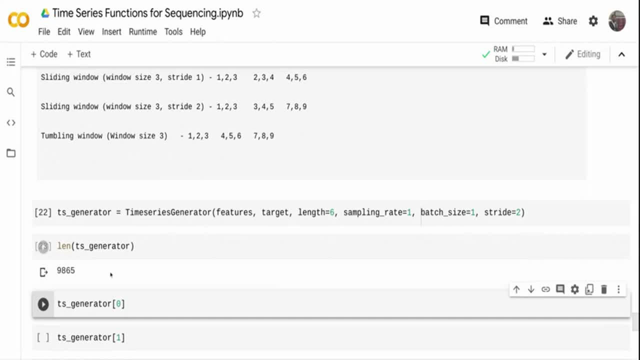 I can print the length of generator. Now, the length, the length of generator will be off of it. Why? Because we are skipping a window, right, That's why stride equal to two will do, And I can print the generator output. 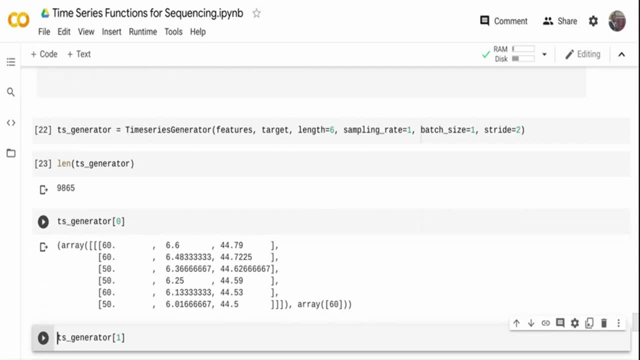 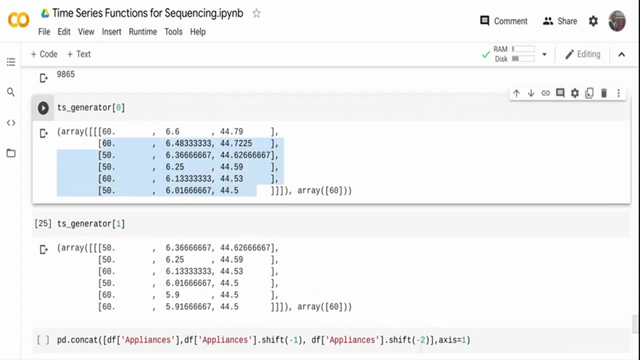 Now, if you see, the first generator will be same as earlier, but the second generator will skip. If you, earlier it was like 60,, 60, 50, it was skip using this one- 60, 50, but you can see it starts from 50 now. 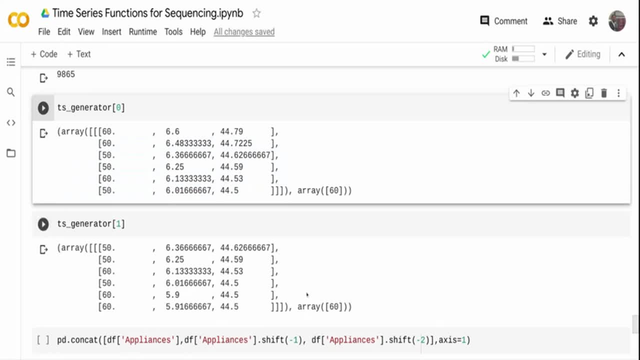 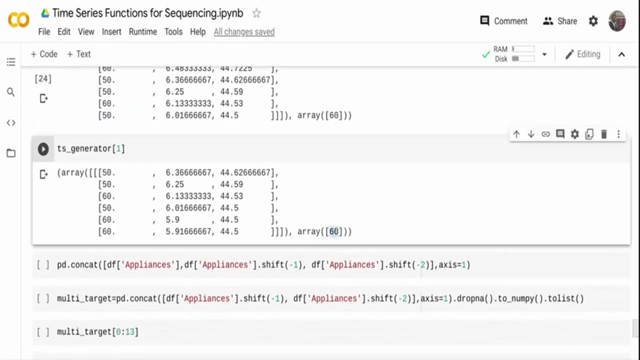 So it's using the third one, So it is skipping the 60, 50 combination, right? What we can also do is now we are only single output over here. If you see, over here we have exactly only one output Now. 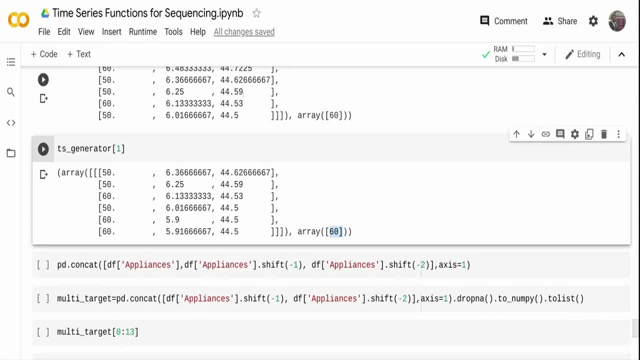 what if you want to predict multiples times? they said so. I want to take T zero to T five. I want to predict T six, T seven, T eight. How can we prepare the data for that? So now, what I'm going to do is I'm going to- uh, first, um the first, prepare my data frame, right? 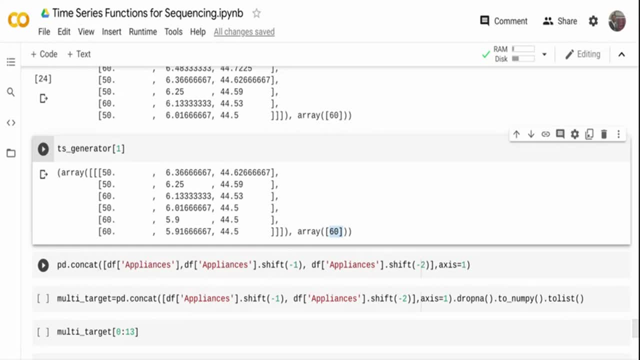 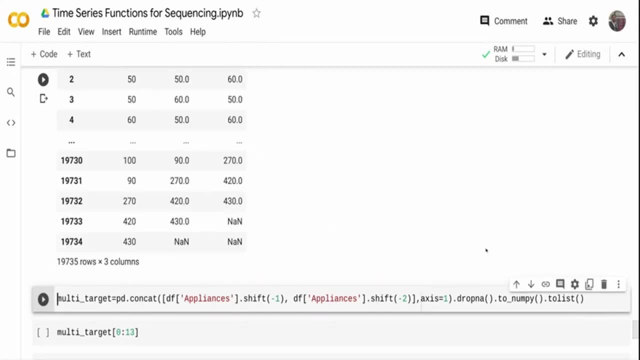 So what I'm going to take, I'm going to take my target appliance. I am going to take appliance and shift minus one and shift minus two. So what it will do is, for each of the value it will give me the next value. 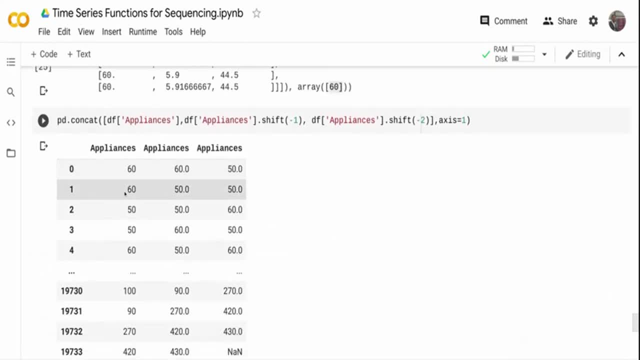 So, for example, if you take here, I get 60,, 60,, 50,. so 60 is my T zero, T one, T two. So when I say shift of one, it's going to take the next value and give me as column. 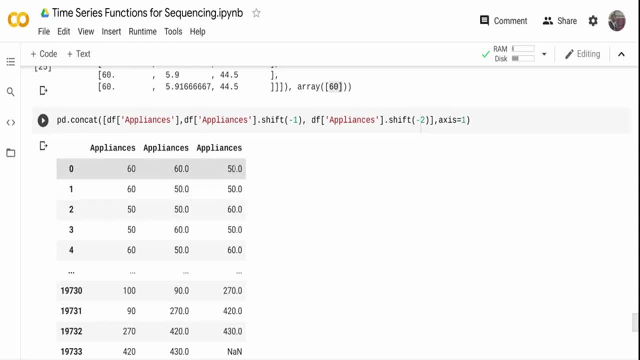 When I get shift of two, it's going to take me a third value as giveaway and give us column. So it's going to do for each and everything over here, each and every row, I'm going to add the current value, I'm going to add the next value and the next value. after that, 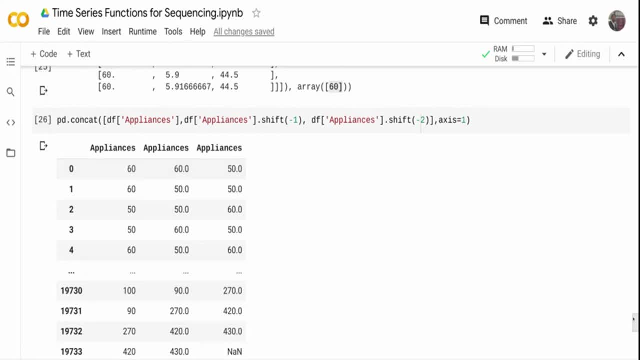 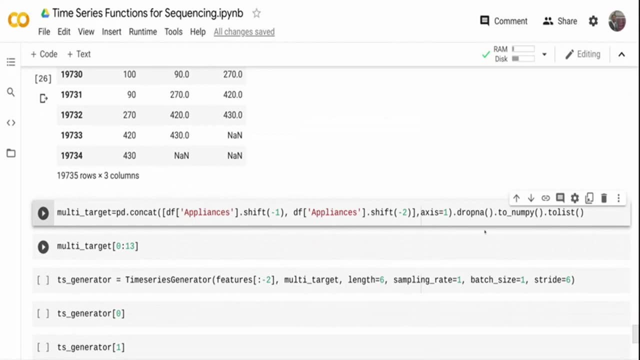 And these three values are the one we are going to feed it as target. So once I have this, I'm going to assign this to an uh variable, I'm going to add a variable called multi-target and I am also telling, like: drop the NA, because what happens when we move uh, when we create the shift right, last row will not have shift when it's C here. this shift of one after this 430, there is no value to have nine and this shift of two after this 430 do not have value. 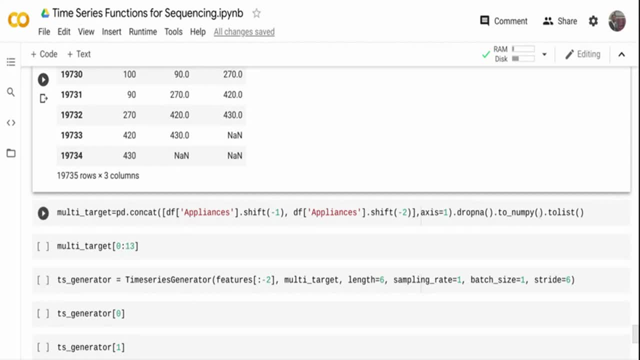 So it will be nine. So I'm going to drop in a, I'm going to do a, two number and two lists. Same as above, same as what we did late me earlier, Right? Um, once I have this: if I print the multi-target, 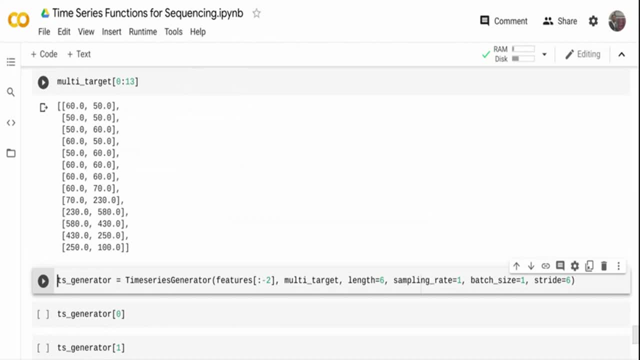 So now I have multiple target value in the appliances. I have like, um, basically, uh, the the next two value over here, zero, one, two and everything. Uh, just one minute, Yeah. So, uh, maybe I missed the DF of appliance. 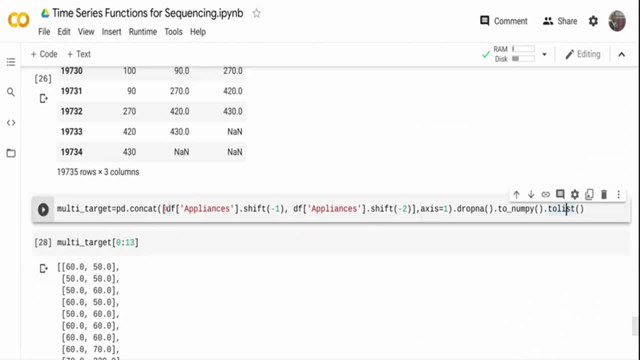 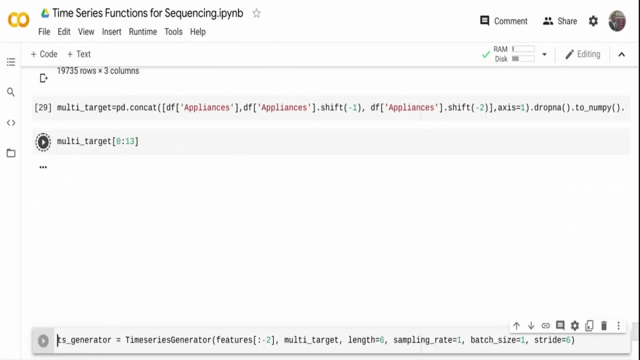 I'm using only the two values. I forgot to add the DF of appliances. so I can do that. Just give me a minute. Yes, I can have that also over here, And then we can run this, and then we can run this. 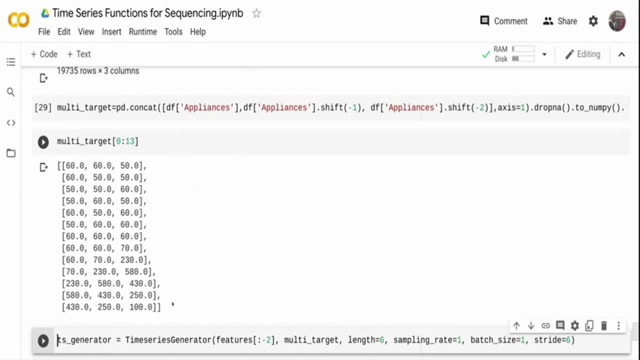 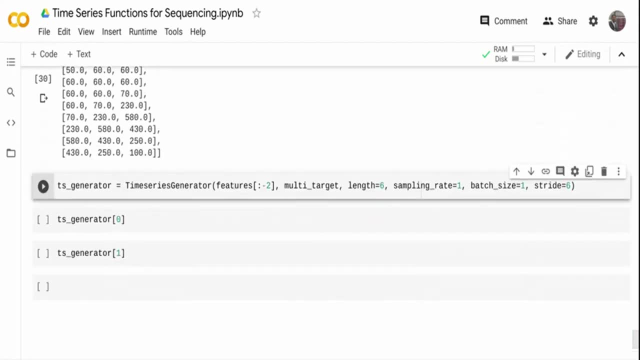 So I will have three values now: 60,, 60,, 50, and all this values I have. now. what I can do is I can go to my time series generator Now, uh, in this case, what I'm doing is I'm taking all my features in the feature, since the last two was in a right. 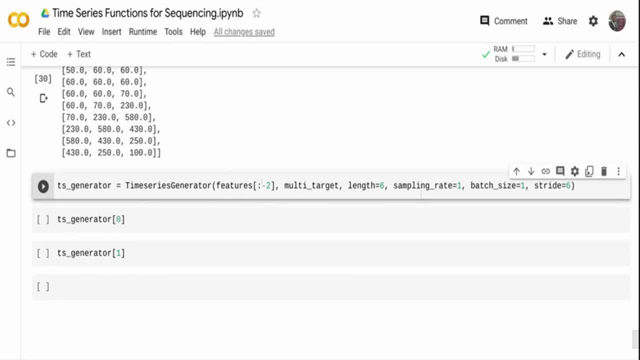 Uh, so what I'm doing is I am basically, uh, ignoring the last two feature column, also because my feature size and the target size as to Match, because I'm doing shift of minus two and telling, ignore the last two colors because I don't have a label for that. 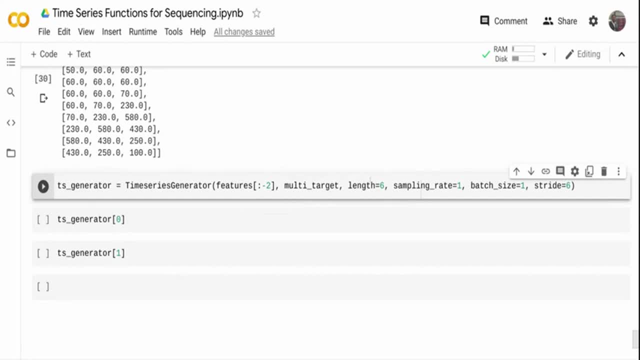 And I'm giving my multi-target over here. I'm giving length as six and telling this game the same sampling rate basis And I'm telling stride as six. in this case, what I wanted to show is the opting window, or tumbling window, because I'm giving length as six and the stride at six. 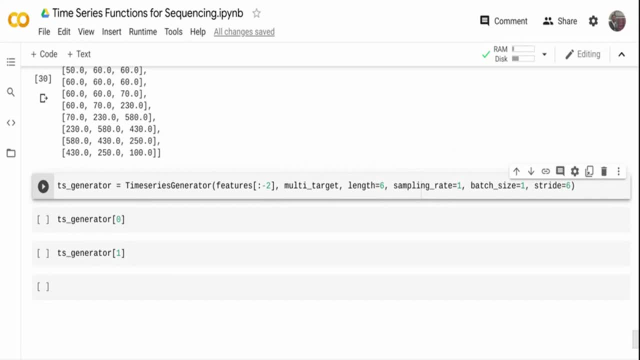 So every time the uh customer will move after six. So this becomes a tumbling window or opting window concept that I explained. So let me run this And let's uh see like all the generator is generated in this case.